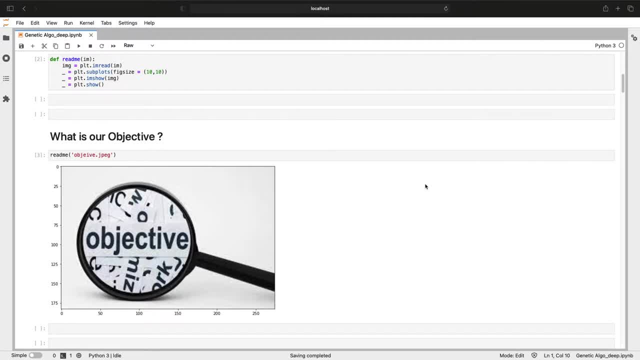 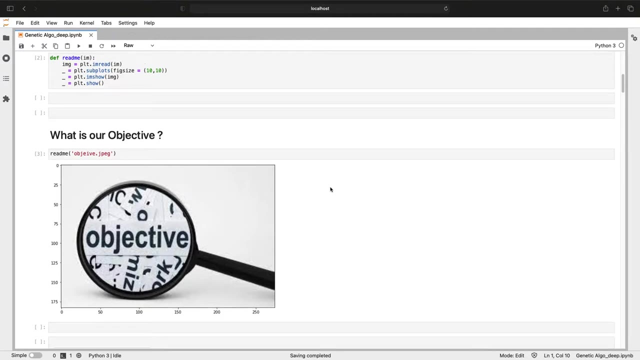 what we are going to do with our production. Like, is it we are going to maximize our production and maximize your sales, or minimize our production and maximize your sales? So we need to have such ideas to write the genetic algorithm. okay, So objective needs to be very clear, okay. So once you have your objective, we need to know. 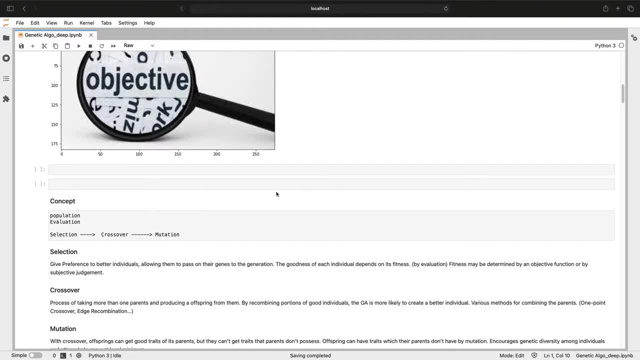 basic terminology associated with the genetic algorithm. One of them is population Genetic algorithm. begin by initializing a population. This is typically done by generating random numbers, and those random numbers are known as chromosomes, and also each individual chromosome is known as genes inside it. okay, So, and the second terminology, what we have? 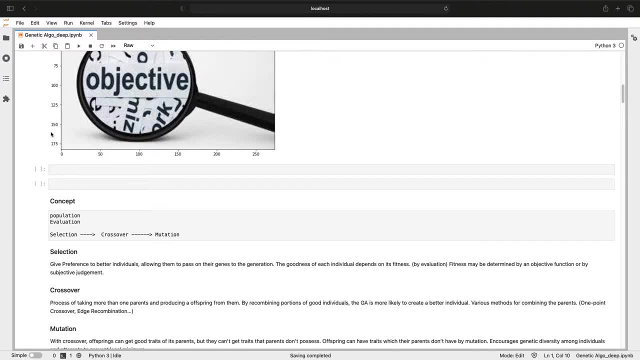 is the evolution Once we have the population initiated. the next the population is evaluated by assigning of fitness value for each of this individual. So, after evolution, the algorithm decides whether it should terminate the process, Depending on the termination condition. what we provide, because the algorithm has, because you 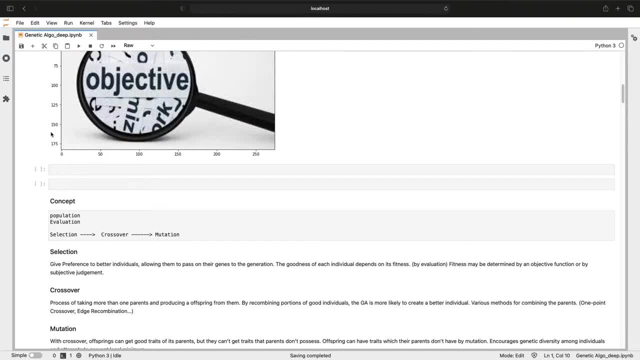 know it might have reached a fixed number of generations or it might have got an adequate solution for the problem statement, what we have defined. So when the termination condition is finally met, the algorithm will break out of the loop and typically it returns its final search result back to the user. So this process is known as evaluation. 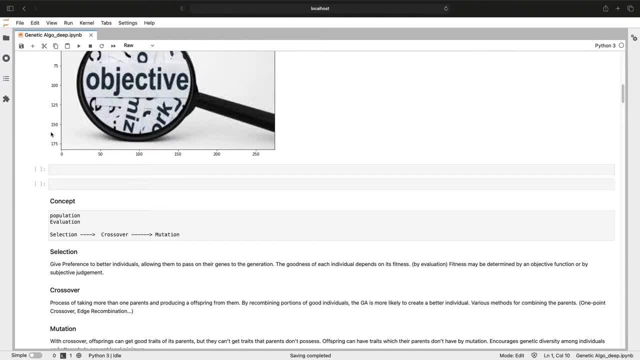 and the next process, and the important one, is known as selection. So let's say the termination condition is not met. right, then the population goes through a selection stage in which individuals from the populations are selected based on their fitness score. So each individual is having a score. 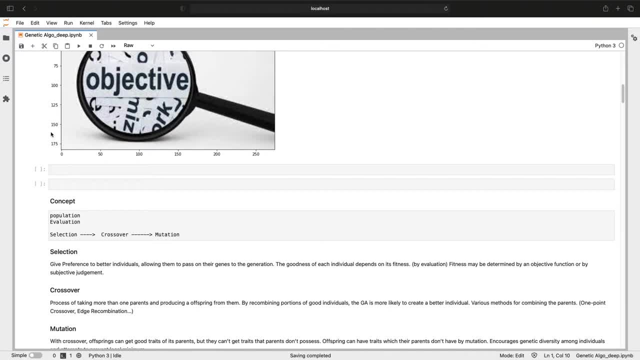 and that score is provided by the evaluation function. Based on the score it is going to select our populations: the maximum the score, the good the population is, And in that way we will be selecting two populations for the next process. So our next terminology is going to be crossover. So basically, crossover is a process which is applied. 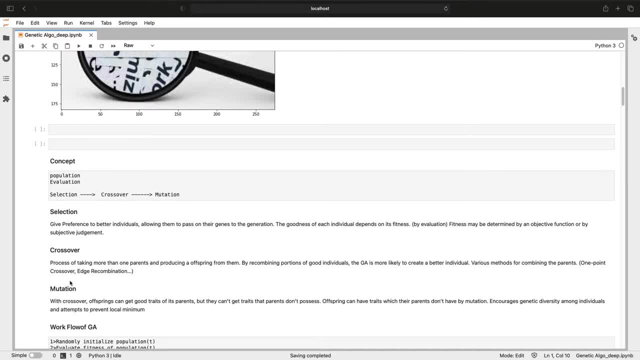 after selection process, and in this process we switch the features of each individuals we selected in the initial processes, right So? after crossover, mutation is going to apply. at this point, the new population goes back to the initial process, So the process starts again, right so? and mutation also creates new values and it adds new features. 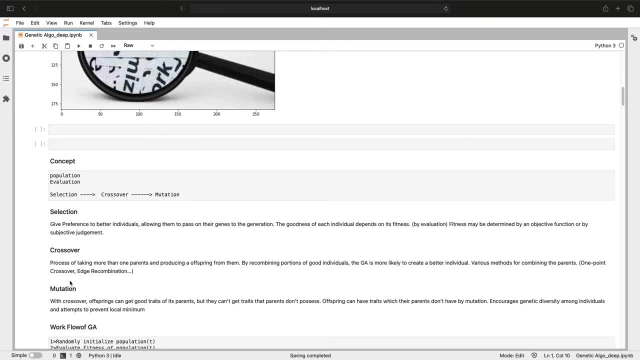 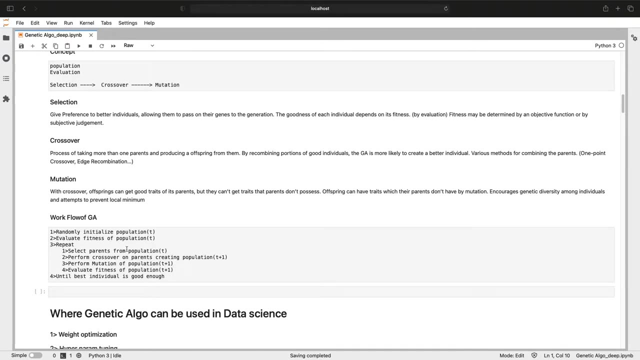 inside our individual and then it evaluates and check whether the new individual, whatever is created, is good or bad, with the help of evaluation process. So the whole workflow of genetic algorithm is going to be like: first it randomly initialize some of the population, then it, then it evaluate the whole population with the evaluation function or the fitness function. what? 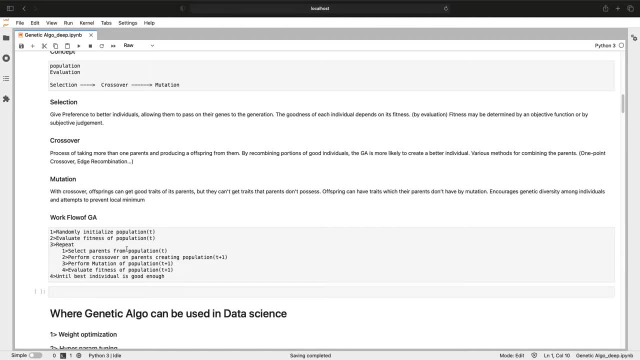 you can say: then a selection process, then crossover, then mutation, and then it again evaluate the new generation, what is generated through these processes. okay, and this whole process of selection, crossover and mutation is going to be in an iterative way till the time it made our conditions. So we need to hold on to this thought. once we look at the code, i think 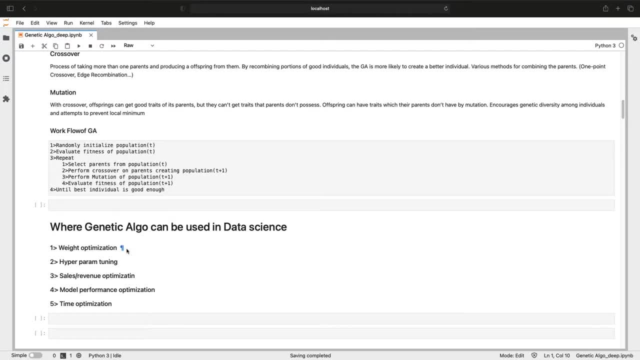 it's going to make more sense to us to where genetic algorithm can be useful in data science. So whenever you are doing any weight optimization or hyper parameter tuning, you can use genetic algorithm flawlessly. so this algorithm is going to give you a good result if the problem 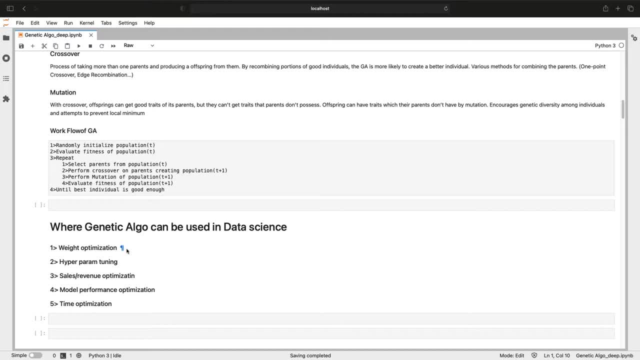 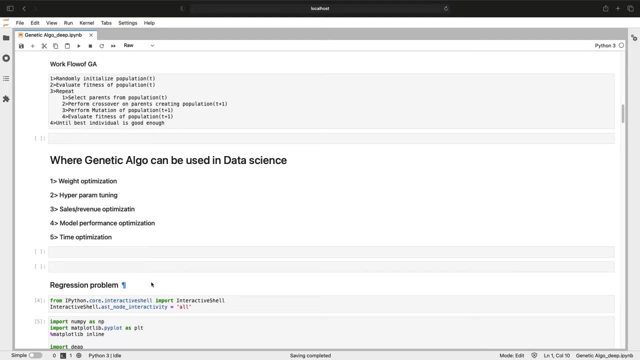 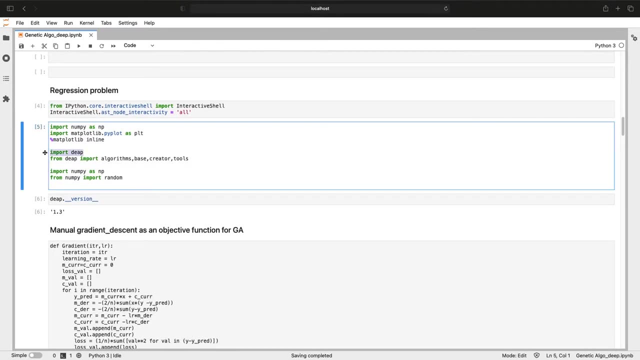 statement is more complex and non-linear. for linear we have lp optimization kind of stuff, but if it's non-linear then we can use this algorithm. So, guys, if we look at the code, for example, purpose: i have taken regression as a problem statement. i have used deep module to write. 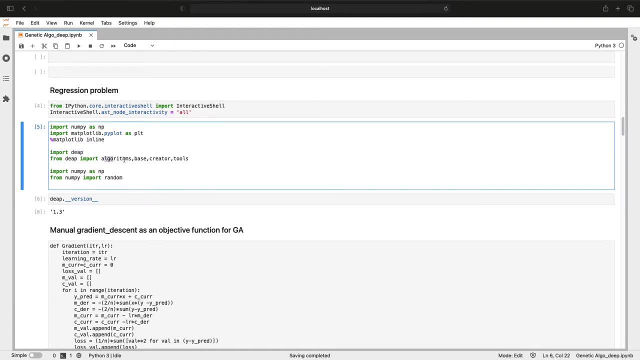 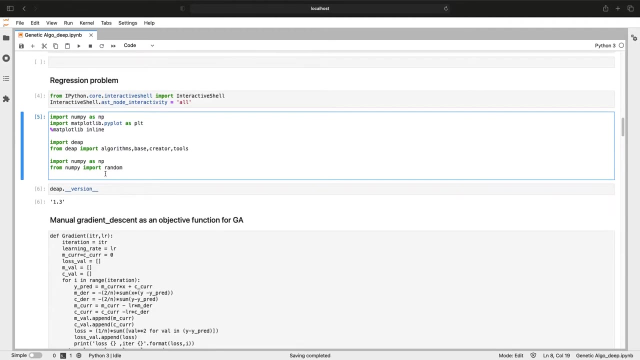 the genetic algorithm and from deep i am using algorithms, base creators and tools module which is available inside it. so from deep i'm using the algorithm base creator and tools and of course, i'm using numpy for some basic data manipulation. and the version of deep what i'm using is 1.3. you can. 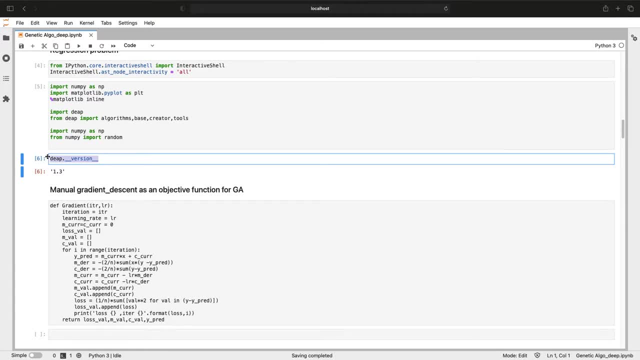 get this specific version from numpy pip or from conda as well. so, as we know, the underlying algorithm used by regression is gradient descent. so the whole intention of gradient descent is going to, you know, optimize the equation of line which is y equal to mx plus c, in such a way that, if you plug in the value of x, 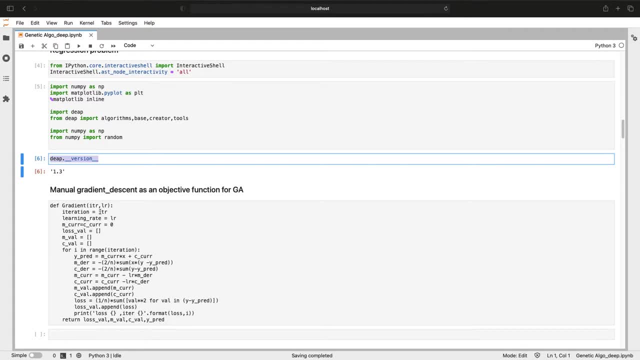 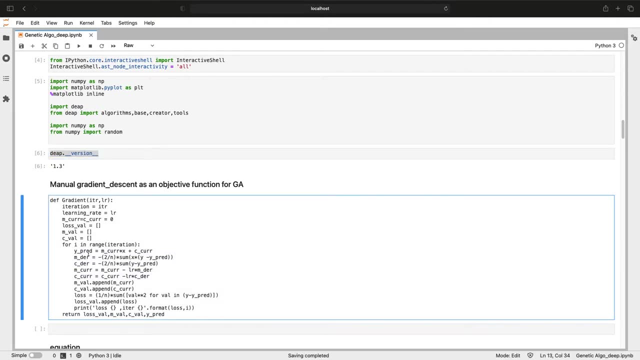 and if we know the value of m and c, it is going to return the value of y. so if you look at this code i have written manually for gradient descent. we have the equation of line y equal to mx plus c and we are calculating m and c through the help of derivatives and then we are updating the m and c. 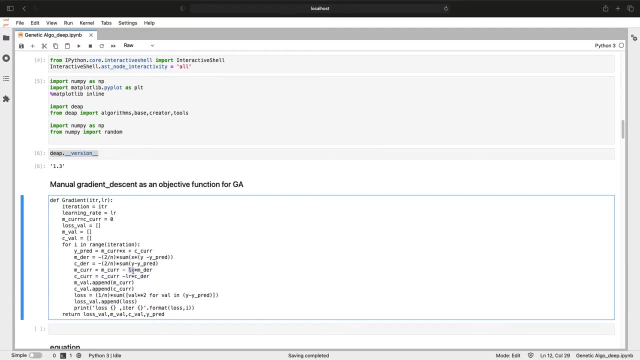 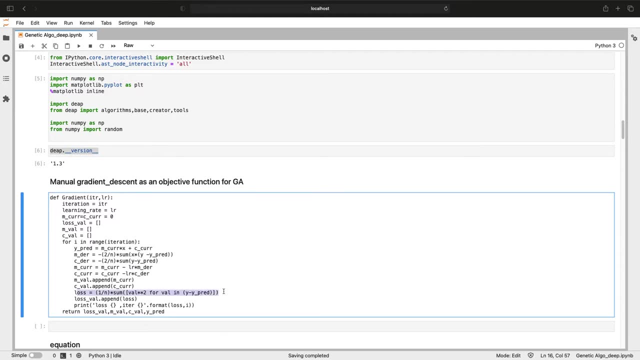 with the direction and step size, known as learning rate. okay, and to evaluate the change of m and c, we have this loss function. so this loss function decides whether the change is good or bad for the gradient descent. okay, but in our example we are. we are not going to use derivative in place. 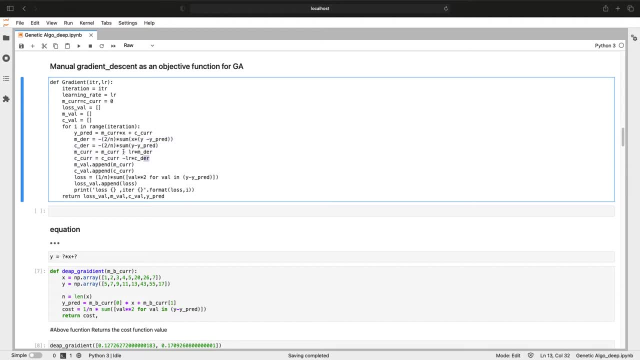 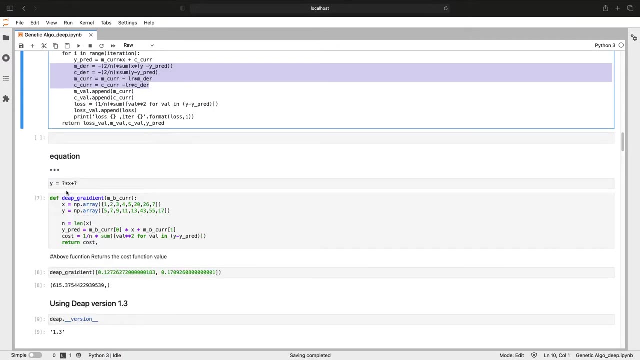 of derivative and updating the weights. i am going to use genetic algorithm which is going to take care of this process and it is going to generate the value of m and c in such a way that it fits, that it, you know, satisfies our equation. so, uh, so now, if you look at the value of x and y, 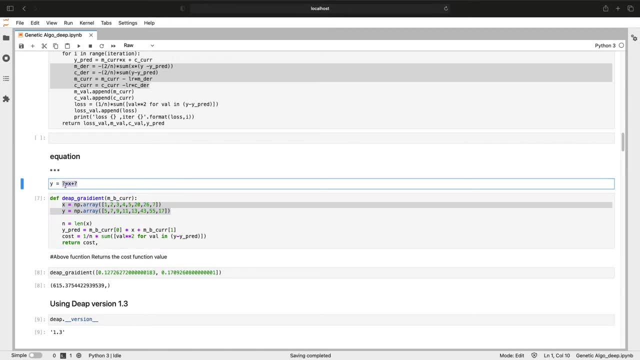 what i have done is i have a equation. we don't know the value of m and c in this specific equation, but if the value of x is given as 1, i need the output as 5. if it is 2, i need the output as 7, and similarly, if it is 7, i need the output at 17.. the whole intention of this exercise is to 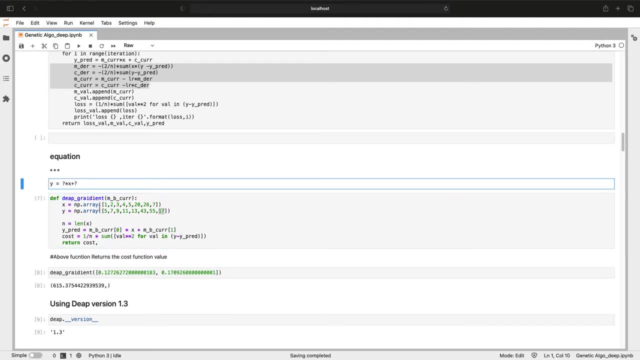 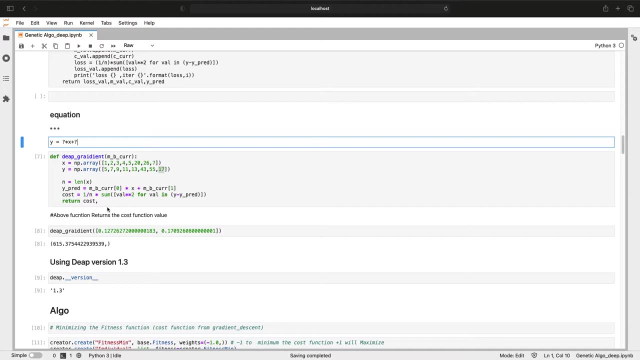 find the value of m and c right, and we can. we are using only genetic algorithm to get those values. so, guys, as i said, objective needs to be clear. in this case, our objective is minimizing the cost function right, because once we minimize the cost, then only we will be able to find the best value. 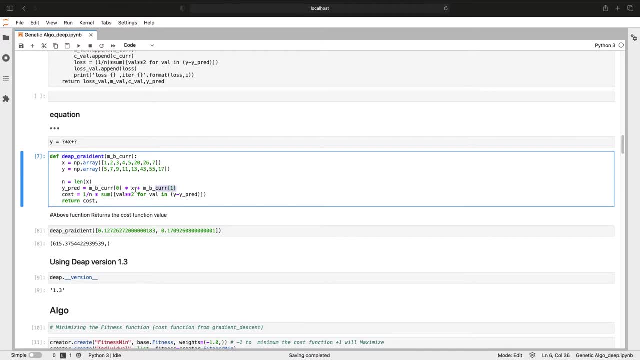 of m and c, which is going to which, if we are going to plug in to this equation, we can get this right. so, uh, here i am passing m value and c value as a list to this function and the first element of: uh, the list is going: 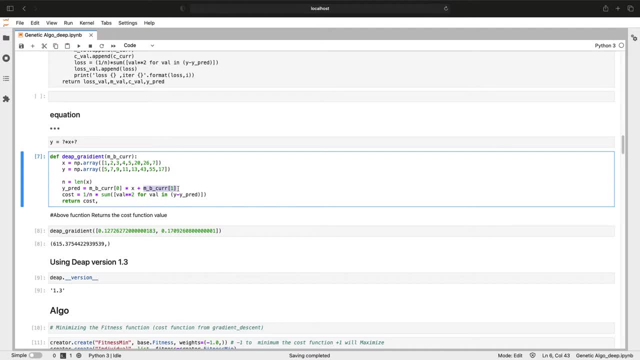 to be m and the first dude lam October 15 is going to be the l of the left point in cambium output. so you will be able to: 2010? 4. wow, i got 1000 points today. bye, bye guys. second element is going to be c. so just to test this function if it is working or not, i have just 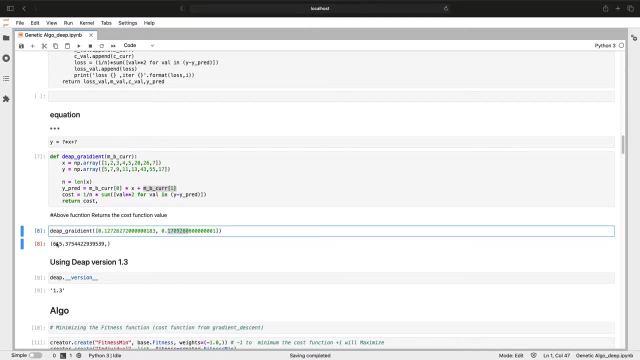 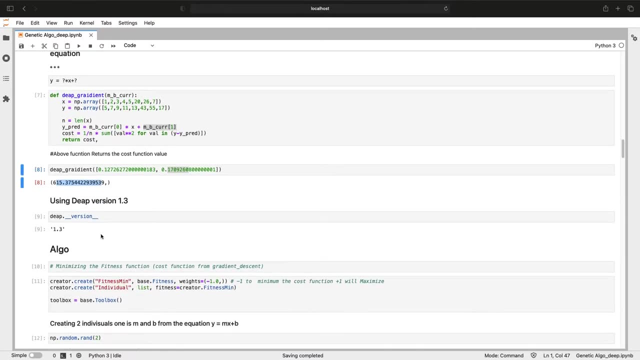 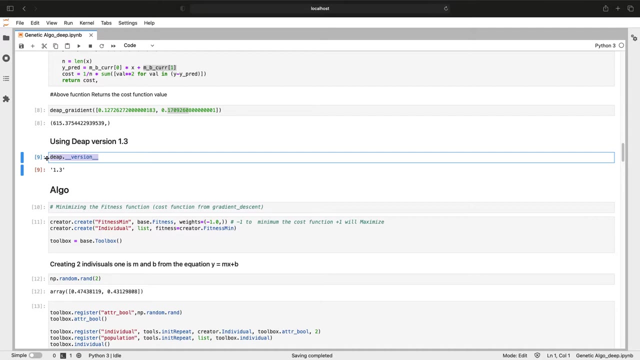 passed two random values inside the function and it is returning the cost function of the loss function inside it. okay, so now we need to prepare the deep module. what is going to give us the best result? so, as we know, we are using 1.3 version of the deep module and the first step, what we do is: 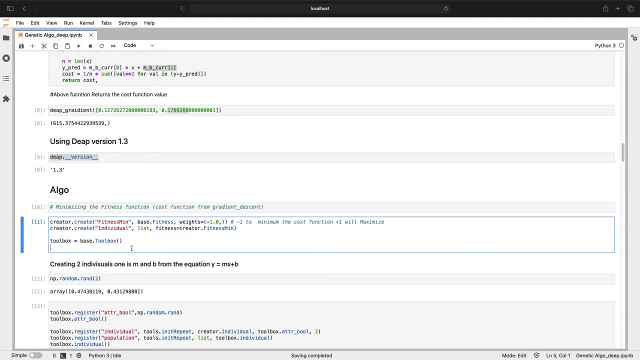 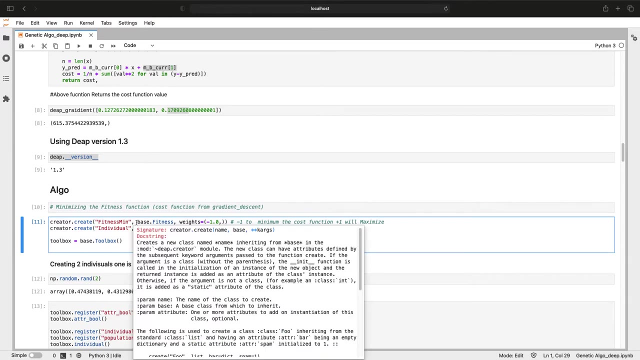 creator. it's a very important tool. so creator basically is allowing to create classes that will fulfill the need of our evolutionary algorithm. so fitness mean is a function, what i'm trying to create right now. so if i'll do ship tab over here i can see creatorcreate. 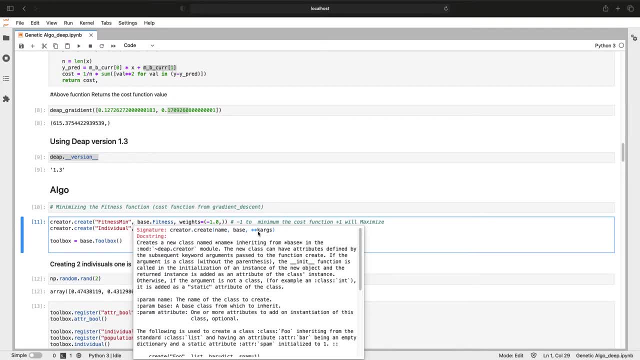 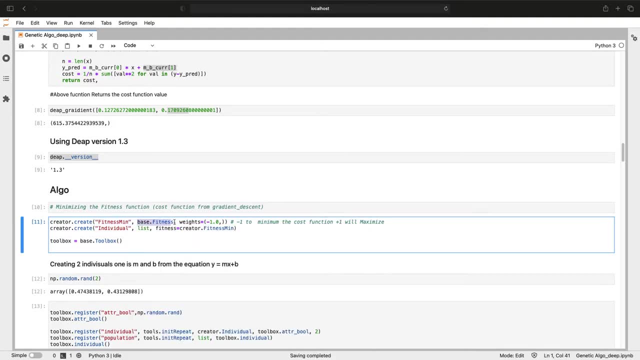 needs three arguments inside it. one is name, base and some arguments. so name is going to be our fitness mean, our base is going to be basefitness, and this fitness needs an argument known as weights. it's either one minus one or so the fitness class is an abstract. 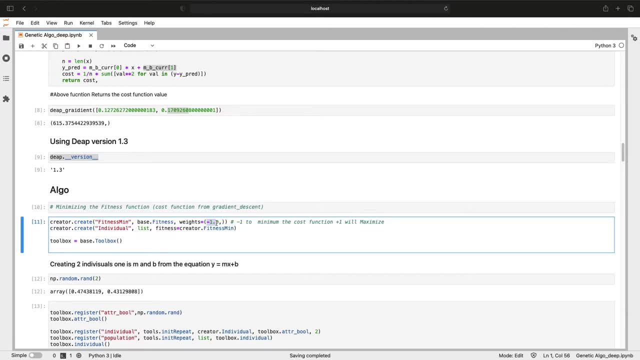 class that needs a weights attribute in order to be functional, and the minimizing fitness is built using negative weights, while the maximizing fitness is built using the positive weights. it means, if you wanted to, if our objective is to minimize something, we are going to use minus one here in this weights, and if our objective 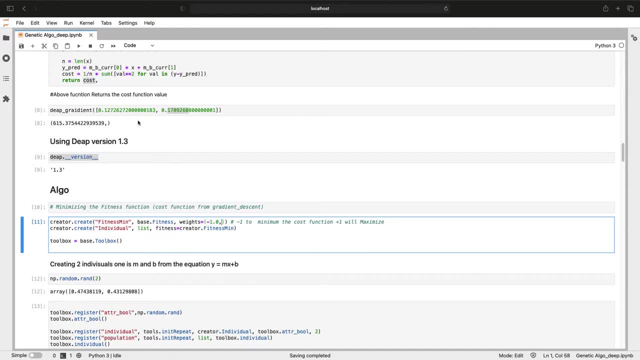 maximizing. we are going to use plus one in this space. but if we have, let's say, multi-objective, like we want to minimize something and maximize something as well, so we need to return those two objectives here and we need to mention minus one and one respective to our return function. 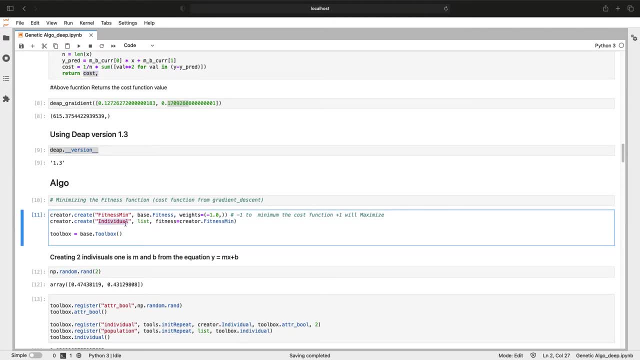 okay, after creating the fitness min, i'm creating a visual function which is a list, and list is going to be a fitness min function. so, basically, i'm creating a list which will be containing all these informations. okay, so what i have done is, again, a toolbox is one more important tool. 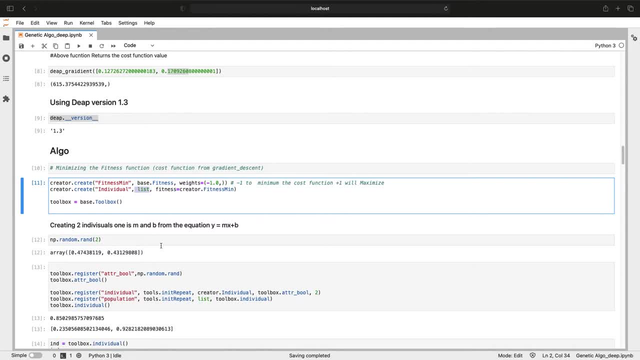 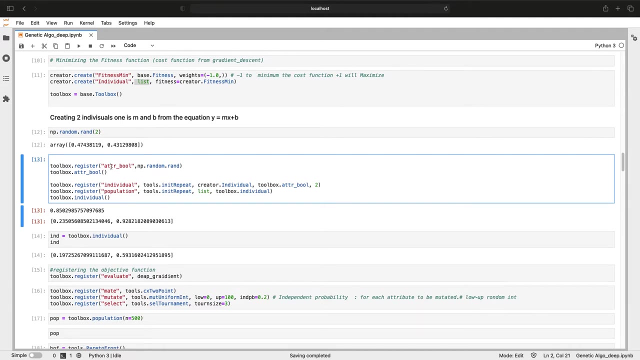 and it is a creator. basically i can say the toolbox is a creator for tools for all sort of action we need in our genetic algorithm and we are going to pass this toolbox to the genetic algorithm itself. so this toolbox need to register all the attributes of genetic algorithms, all the 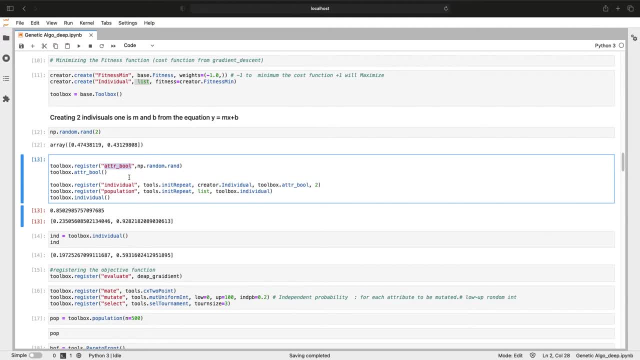 features of genetic algorithms. basically so we are registering all the attributes of genetic algorithms, all the features of genetic algorithms, registering our first feature, which is attribute boolean, and it takes input as a numpy dot, random. so, basically, if you want to create your own attribute boolean, which is which is going to 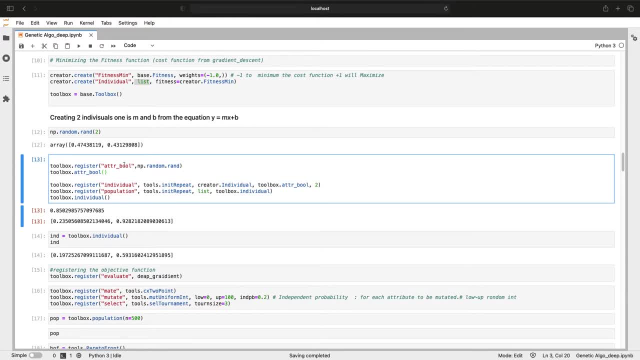 generate weights. you can write your own function and you can pass the function name over here, right. in this case i'm using numpy to generate the random weights. so if you see, if i'll run this attribute boolean, it is going to return a single value, because the default properties of numpy is 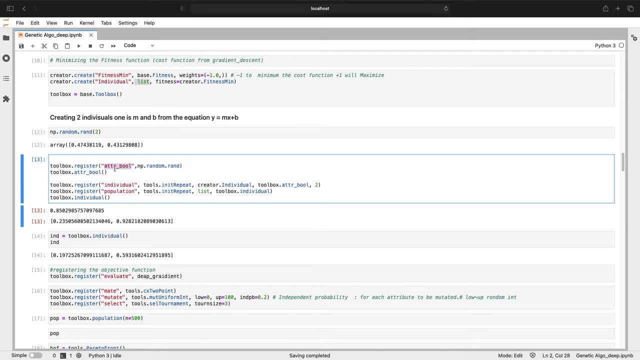 one. so now what i'm doing? i am by using this attribute boolean, i'm creating individual. individual is basically one chromosome, so i'm creating this individual using this attribute boolean. as you can see, i have mentioned attribute boolean over here and i am creating two genes. so, as i mentioned, genes are part of the chromosome and i need two weights to be. 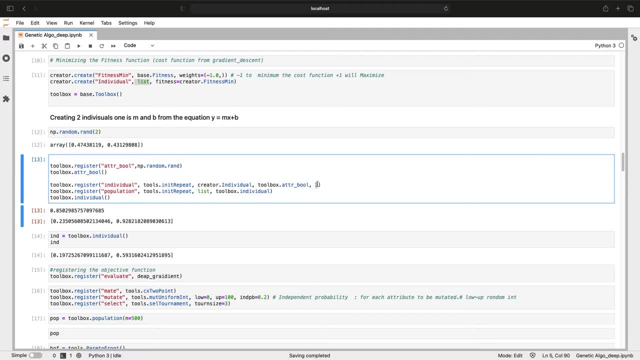 passed to the function. so that's why i need two genes over here, two random numbers, what you can say in computer terminology. so if you see in numpy function, if i pass two here it is generating, it is giving two randomly generated array. so this is what i'm getting here, right, and this whole setup. 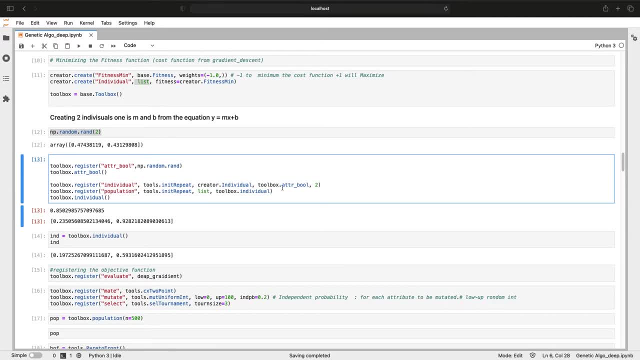 is used by population. so population is basically containing these two informations inside it. it is going to contain a random number. so basically, in such a way, it going to contain an array and the no. in this case, the population is going to contain a list of random numbers and there will 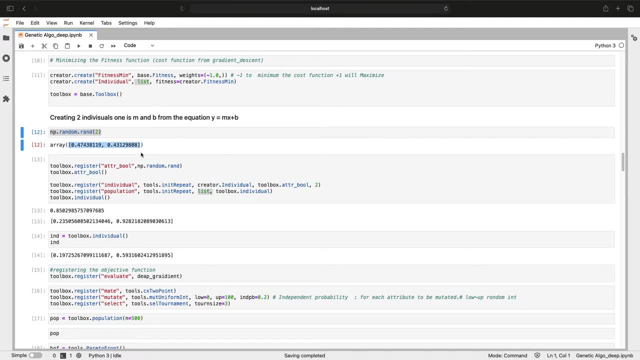 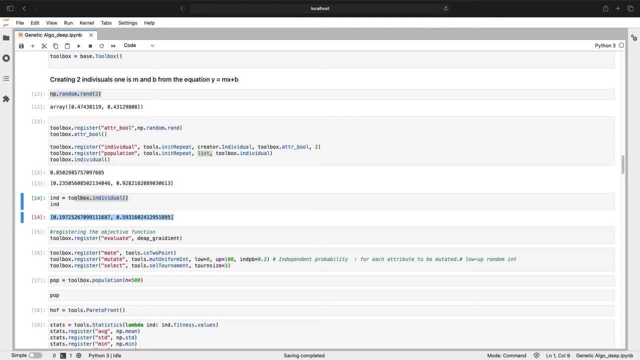 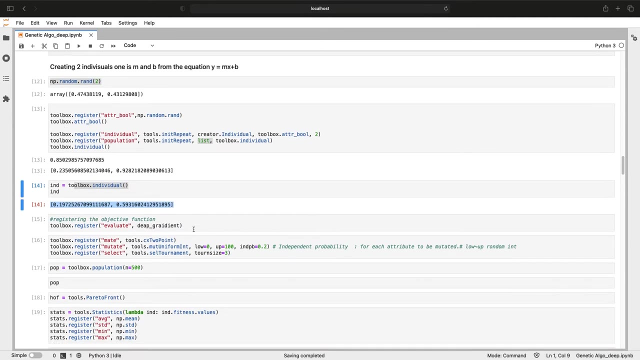 be two random numbers in each and every individual. okay, so now, uh, if we print toolboxindividual, you can see it is generating one set of random numbers. in that way, we are going to create a whole population of these random numbers. okay, so now the evaluation function, as i mentioned, defgradient. 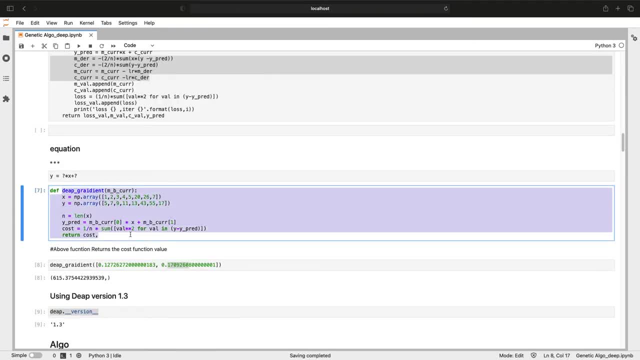 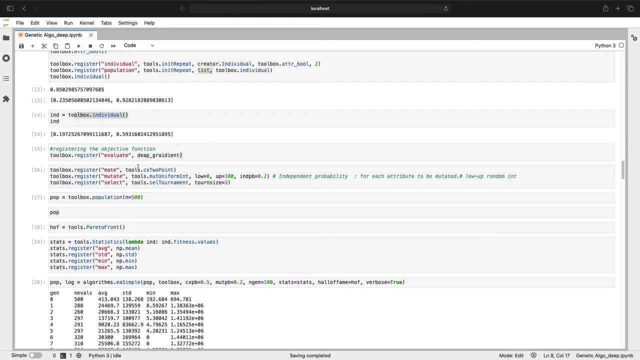 what we have written here. the first step is going to be our evaluate function. so, by using deep gradient, we are going to evaluate how our weights are. okay, once we generate the population, we'll be using the evaluate function, which is alias of deep gradient, what you can say. we are going to use this function to evaluate our 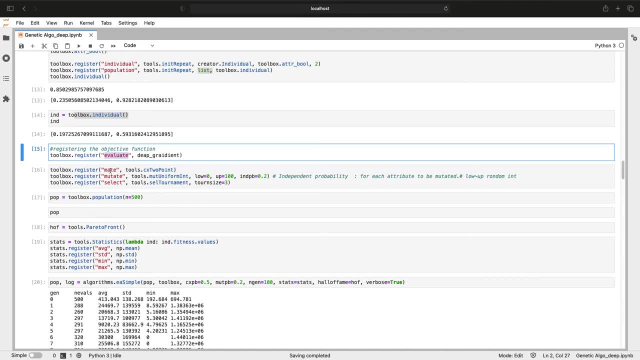 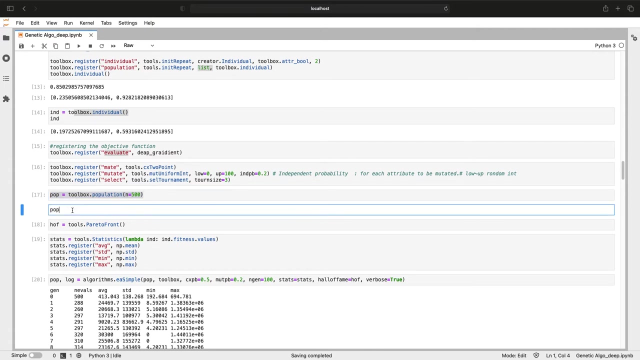 population. okay, in the similar fashion, i am registering mutation, selection, mating and everything with all the information. so i need. these are the default values you can get in deep documentation. it will give you more information regarding this. so, guys, in the first days i am creating a population of size 500. if you run the population it is going to give you. 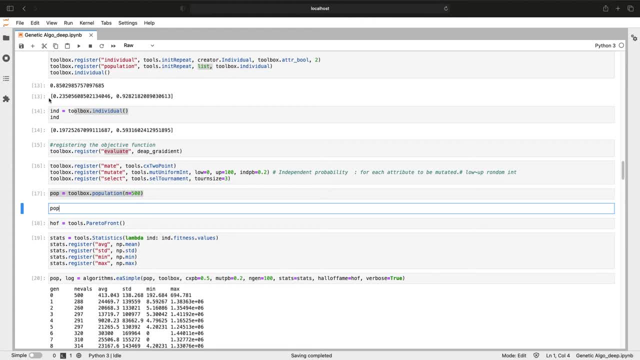 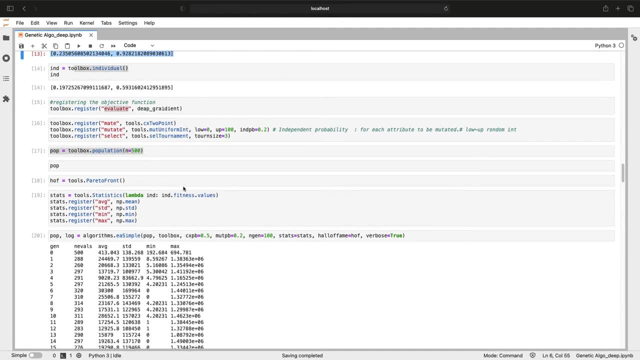 a 500 set of random numbers, and each set is going to have two numbers inside it, so these are going to be the value of m and c. okay, so now you need the name of the population and this will be our. actually, our name is going to be hall of fame. 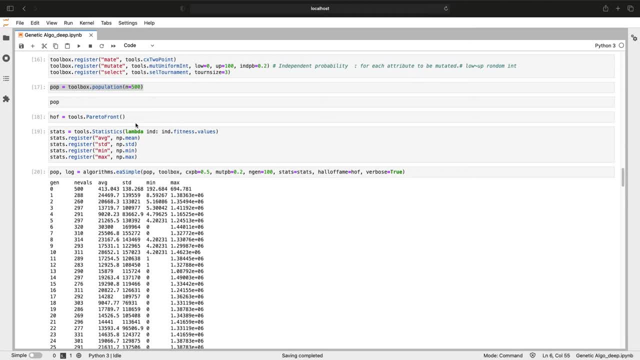 hall of fame is basically a archive. what will store the best results from our population, from each generation, whatever the best result we get? it is going to store that and the stats. it is basically to calculate the statistics and we are going to need this in algorithm. 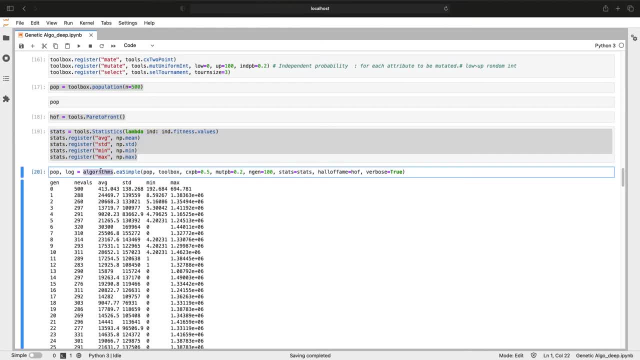 in algorithm modules. so once we so once. so here we have the algorithm model and we are going to. here we are using a sample algorithm and inside a sample we pass the whole population, then we we pass the toolbox, what we have registered here. then we have cx probability. 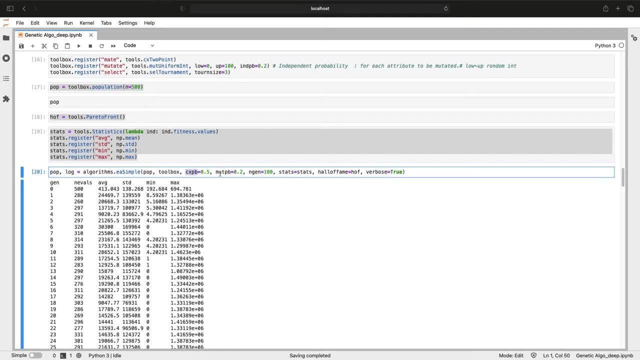 basically cross section or crossable probability, what you can say. then we have the mutation probability and the number of generation is 100. the number of generation is basically what you can think of as a epoch and stats. here is going to be the stats, what we have created. 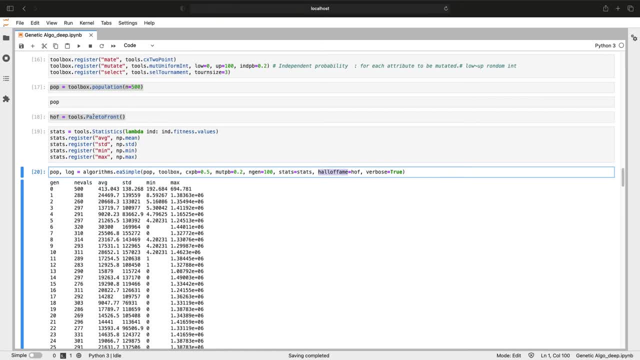 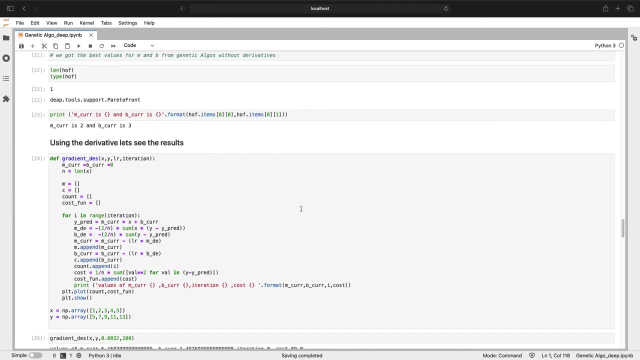 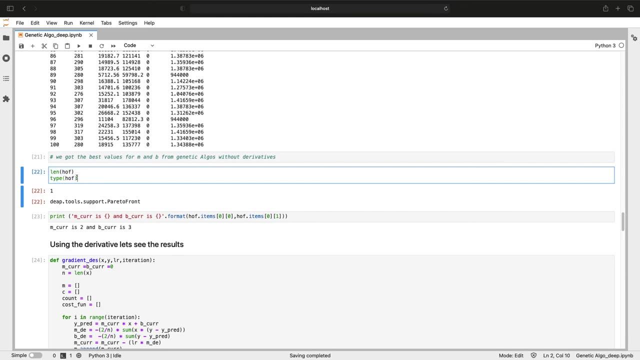 and hall of fame is going to be hof, what we have mentioned as pareto front and, yes, we wanted to see all the information about the model. so once we run it, we will have a hall of fame which will be saving all the good results. basically- and if i see the hall of fame length is gone, so it is it have. 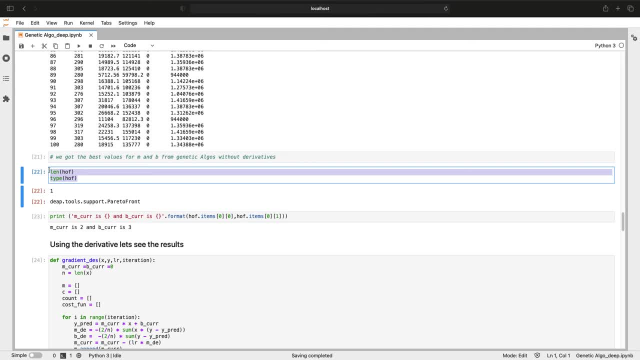 only saved one result, but in your case it can save multiple results as well. okay, so if i print the first elements, first value, uh of hall of fame, it is going- it is showing us two and the second value of all of them it is, it is showing as three. so it means so. it means that genetic algorithm has given us two values. so 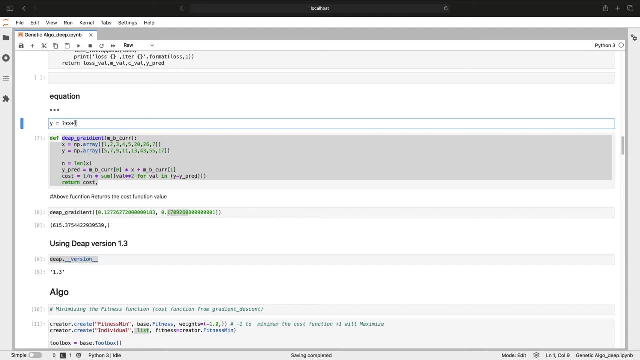 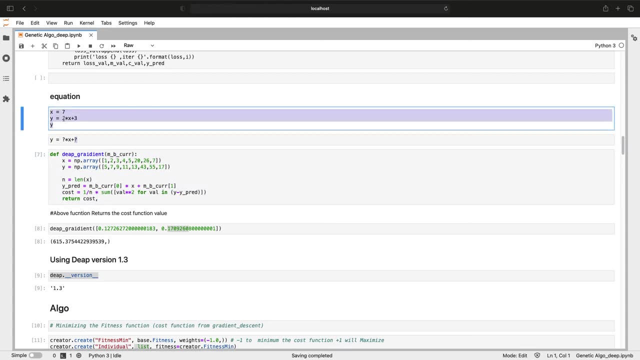 those values if i'm going to put in this equation, it is going to give us the result, what we expect. so now, uh, to generate this value of x and y, i have used this function. as you can see, two and three i have used here to generate those numbers. so now, 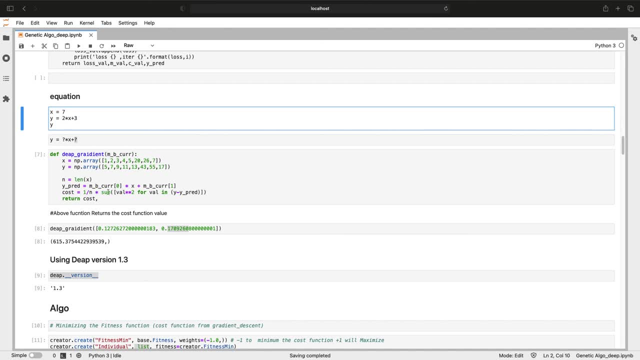 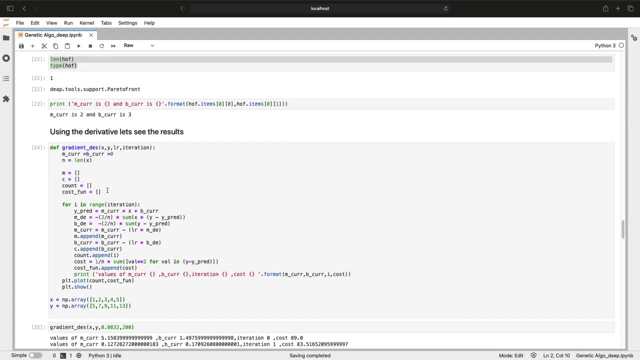 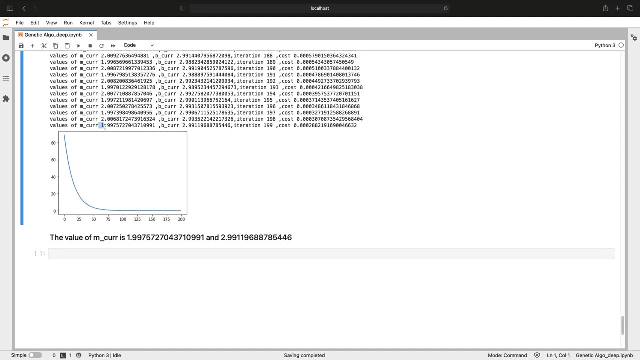 algorithm was able to get those number, get those values of m and c in this case. okay, so i have created a gradient descent, also in the same fashion. gradient descent is going to run with a specific number of iterations and it is also going to give us the same result, almost. 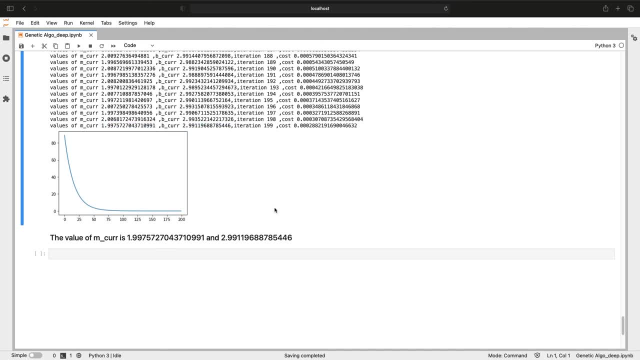 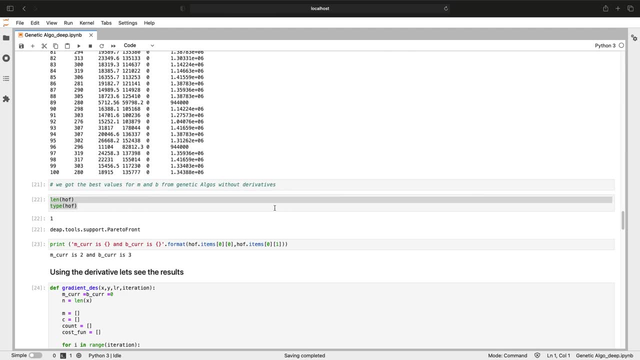 around two and this is almost around three. so, guys, this code you can take and you can use it in your specific use case by changing those specific values i have mentioned, and this is going to be helpful for your complex problems mostly. so, guys, also we have the deep 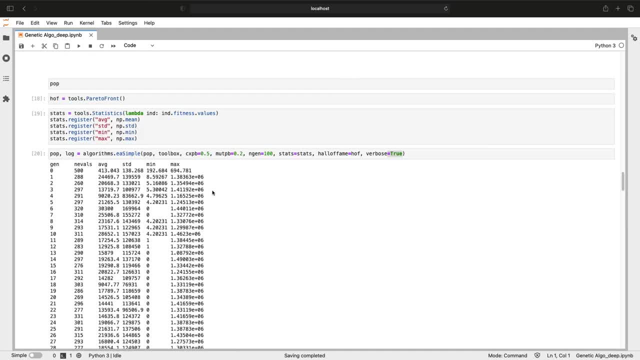 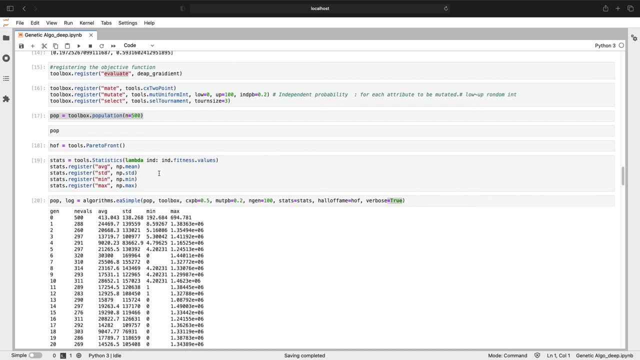 documentation page. if you need to understand in depth of this specific code, you can just go to the deep documentation and there you will get a lot of help out and also like, share and subscribe to my channel if you want to know such beautiful algorithms related to data science in future.